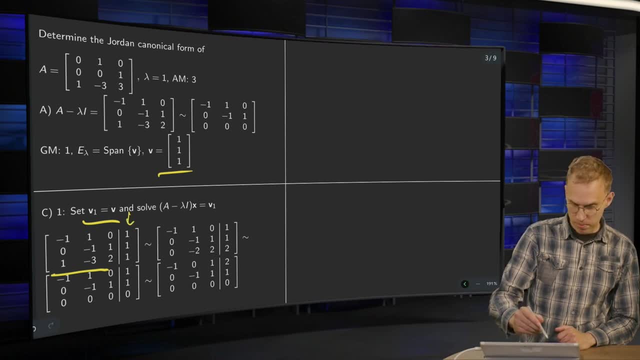 And here we have our V. Do the same row reduction step, Like: add first row to the last one. Then we get 0, 1 minus 3 equals minus 2.. 0 plus 2 equals 2.. And 1 plus 1 equals 2.. 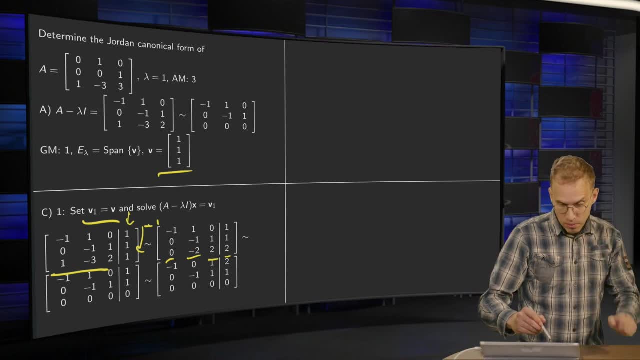 Let's see how do we continue. We subtract the second row twice from the third, Which gives us a row of zeros over here, And then let us add this one over here. Let's go all the way to reduced action form, Which gives us a 0 over here. 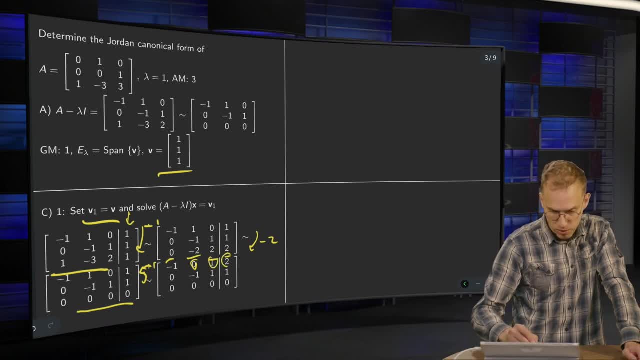 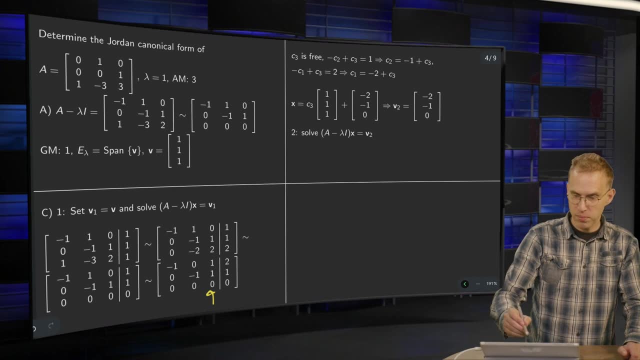 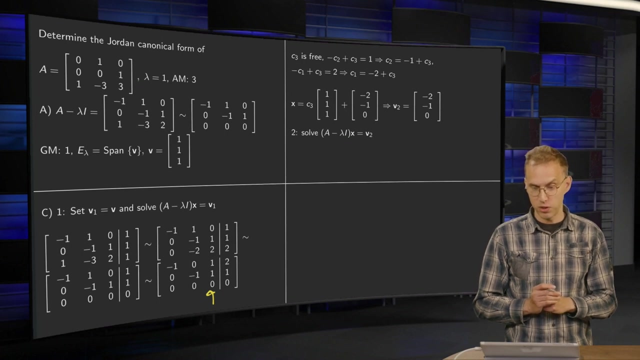 And 1 plus 0 equals 1. And 1 plus 1 equals 2.. So there we go, And then we solve with C. C3 is a free variable. The second row gives me: 0 times C1 minus 1 times C2 plus 1 times C3 equals 1.. 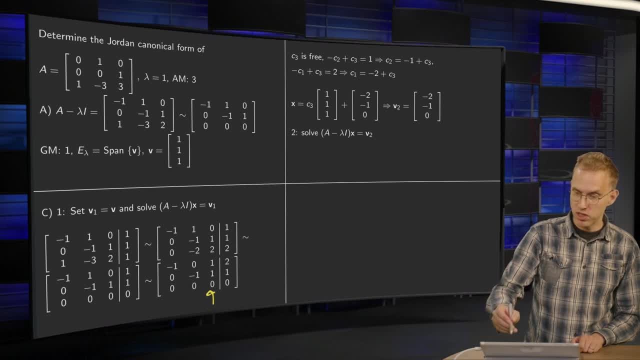 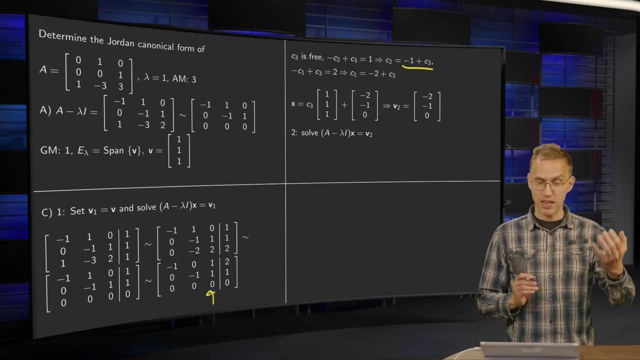 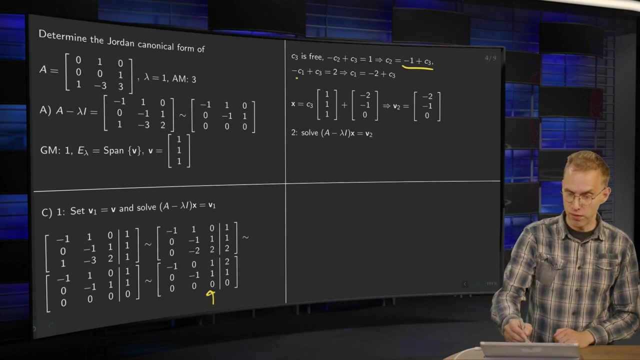 So we can express C2 and C3.. C2 equals minus 1 plus C3.. And then the first row gives us minus C1 plus 0 times C2 plus C3 equals 2.. So we can solve for C1.. 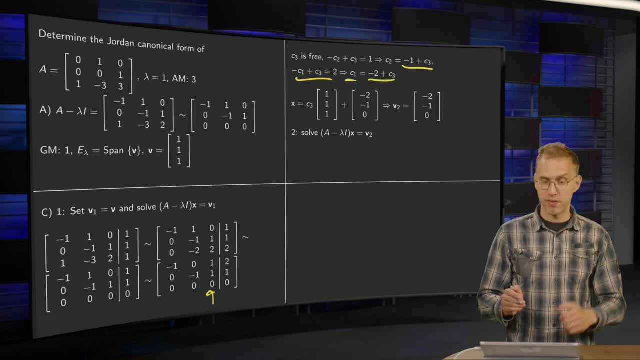 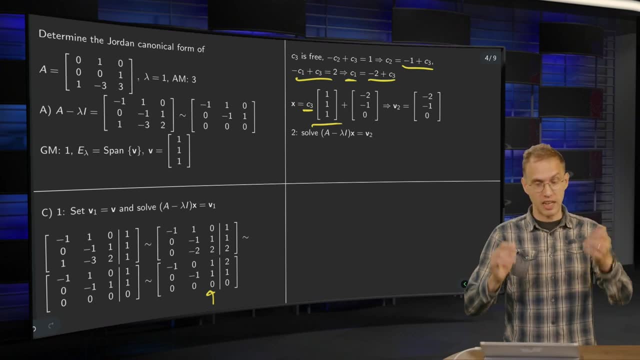 C1 equals minus 2 plus C3.. And we write down the parametric vector form: x equals x equals C3 times. Well, the eigenvector as expected, Plus some particular solution: minus 2 minus 1, 0.. And then we know my second generalized eigenvector. 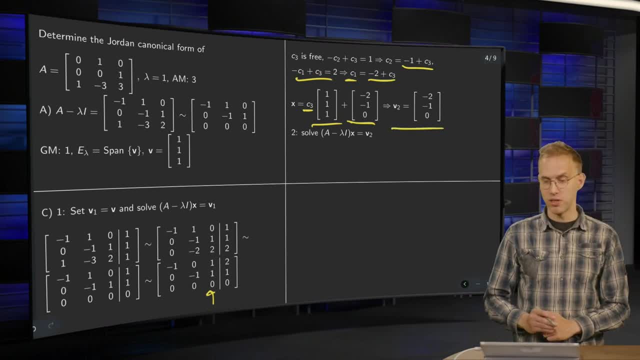 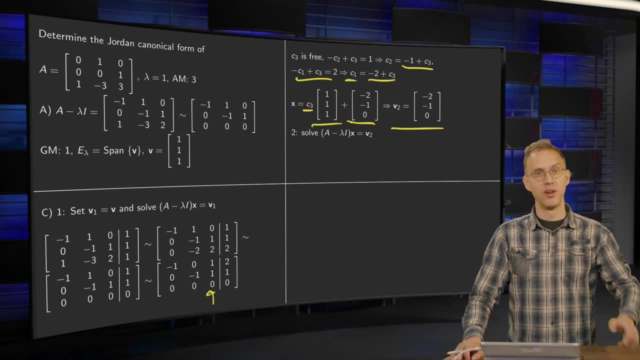 But as we can take the particular solution, V2 equals minus 2 minus 1, 0.. So there we have our second generalized eigenvector. Going on to the third one, We do exactly the same: Solve a minus lambda i times x. 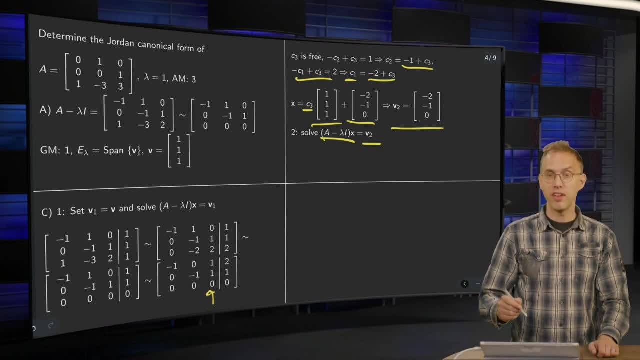 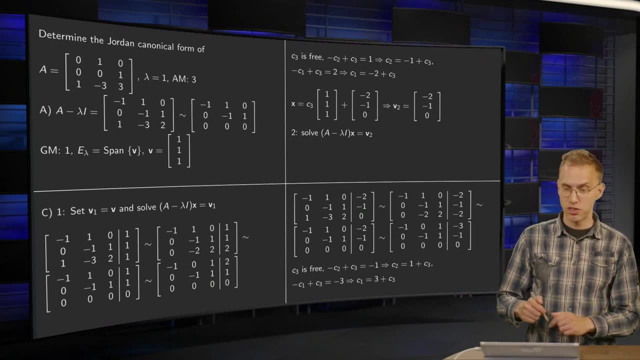 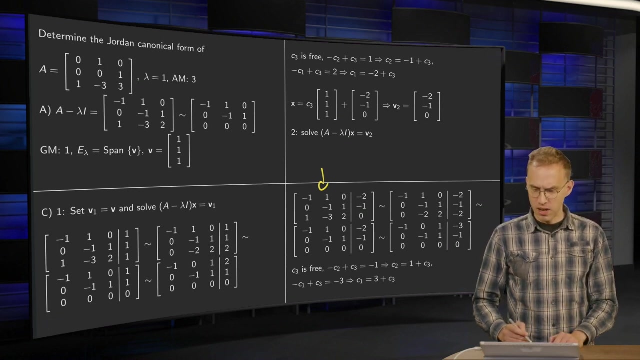 But now instead of v1 we put v2.. So the only thing which is going to change Is that our right hand side here becomes slightly different, So we can do the same row reduction steps. So this part will remain the same, And only the right hand side is changing a bit.